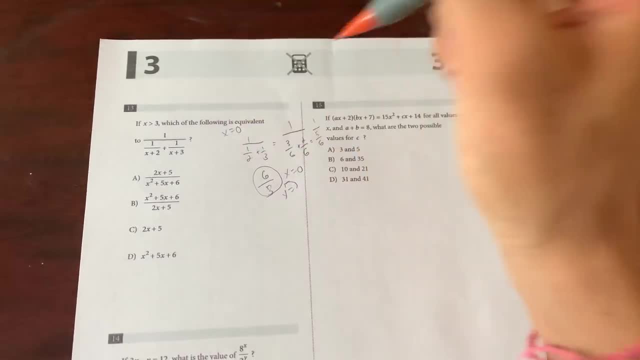 So this is basically an elimination method, And most of the time this eliminates all 3.. So let's plug in 0 to the first one. You get 5 over 6, right, Bang, bang, gone, gone. 5 over 6.. 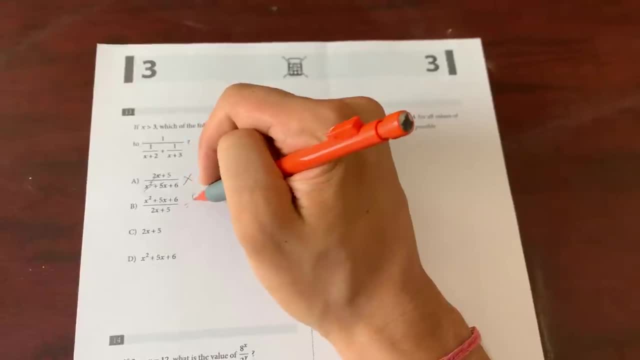 That's not 6 over 5, gone. Plug in 0,, you get 6 over 5.. So this works. So this passes on to the next round. You plug in 0, you get 5.. You plug in 0,, you get 6.. 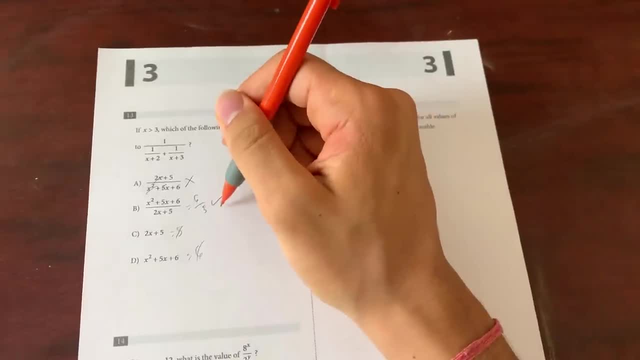 So only one problem passed on to the next round. So only one problem passed on to the next round. So obviously that is the answer. That's the correct answer. 13 is b. So you guys, very simple. 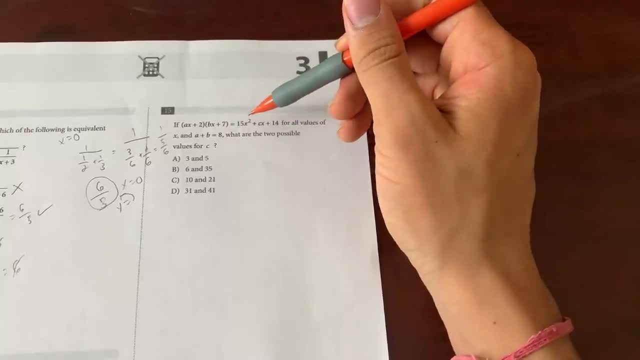 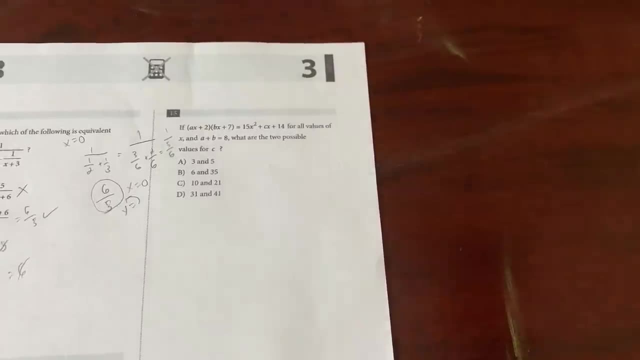 Now this one right here: If ax plus 2 times bx plus 7 equals 15x squared plus cx plus 14, for all values of x and a plus b equals 8, what are the two possible values for c? See, a problem like this is what you see on the SAT a lot. 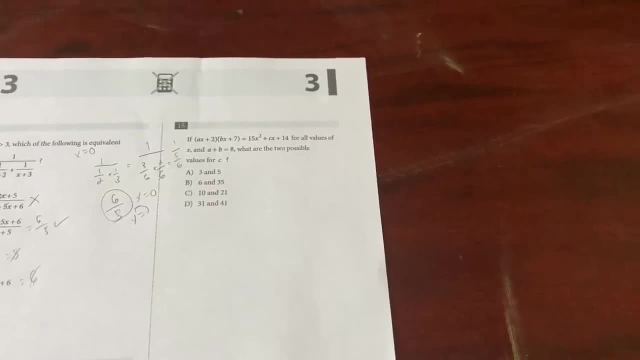 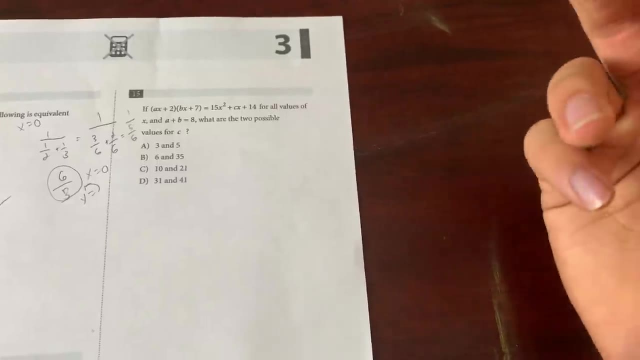 Like it's just worded weird and it's not like a direct question. This is a direct question, right, Just like hey, which is the equivalent. This is, just like you know, worded weirdly, and you're just like: alright. what is it trying to ask me? 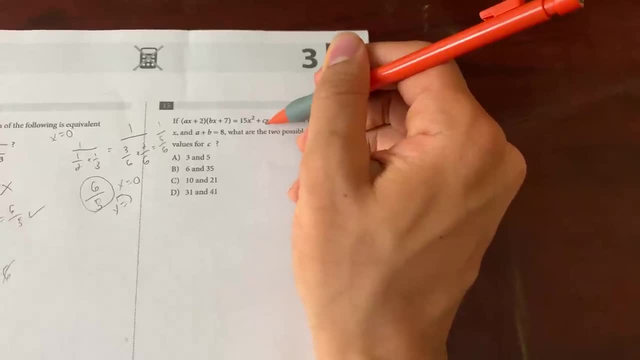 Right. So you're trying to find the values of c, okay, So what this basically is saying is that there's two possible values of c. So you know right now that there can be two possible values of c. So you know right now that there can be two possible values of c. 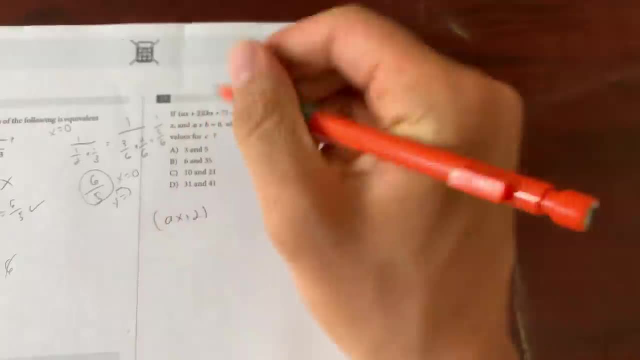 And you know that ax plus 2, see, I like to rewrite the main part. equals 15x squared plus cx plus 14.. equals 15x squared plus cx plus 14.. equals 15x squared plus cx plus 14.. 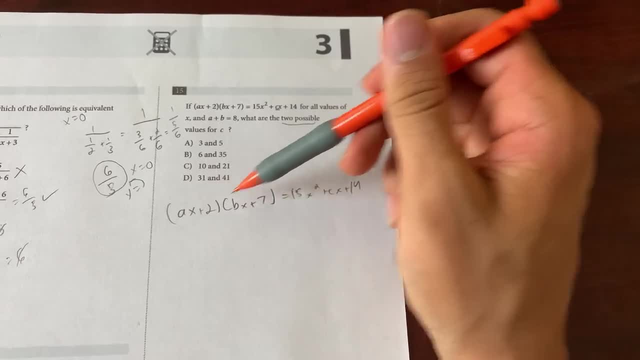 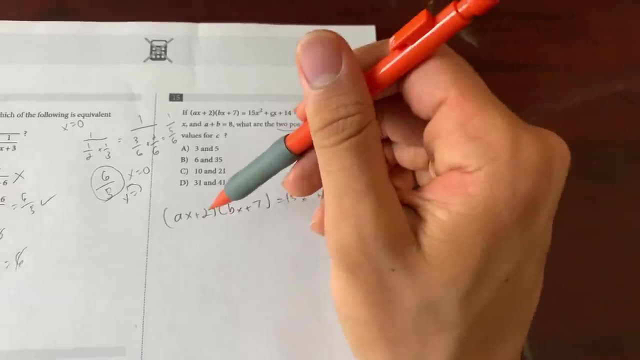 So what is this telling me to do? I'm trying to not factor this out, right, I'm trying to like distribute it out, so you get this Okay. So how can I match the left side to the right side? 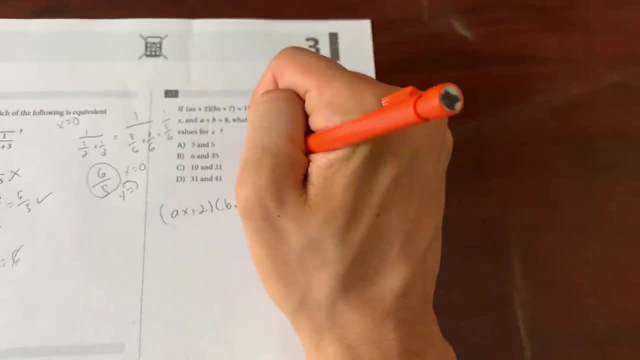 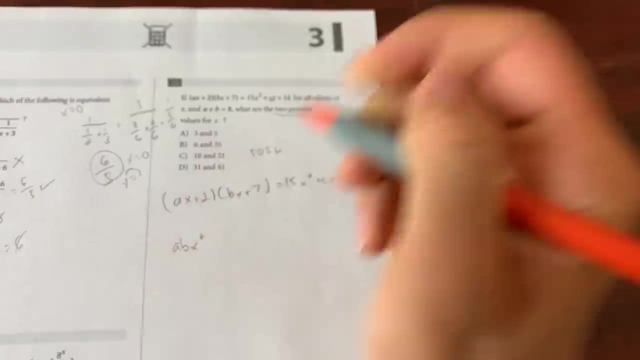 Alright. So I know, if I use FOIL right First, outer, inner, last, The first terms multiplied together, which will give me x squared, which will give me abx squared, need to equal 15x squared right. 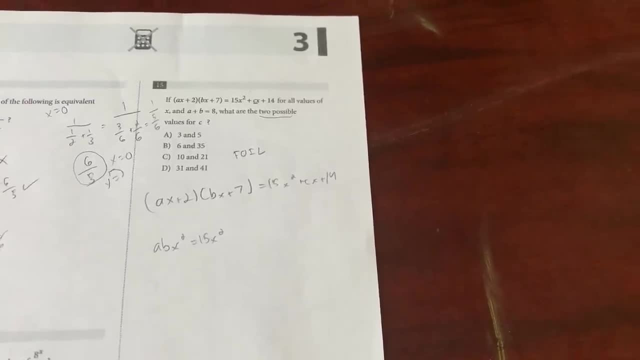 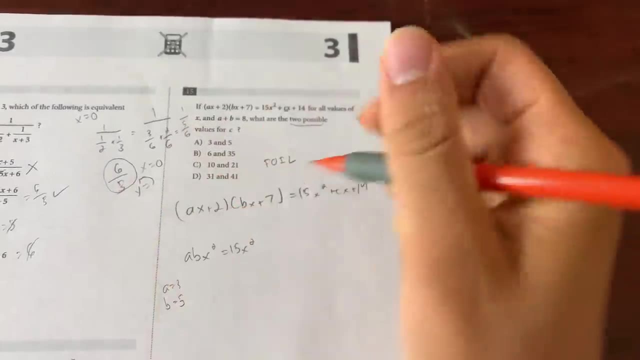 So what can a and b be? Hmm, let's see. Well, what times? what gives you 15? 3 times 5 gives you 15.. So let's make a equal 3 and b equal 5.. Oh yeah, and a plus b equals 8.. 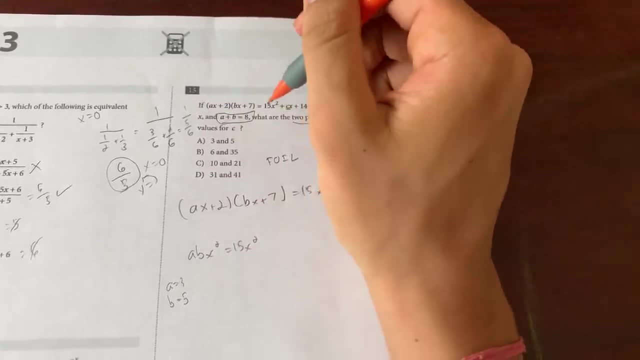 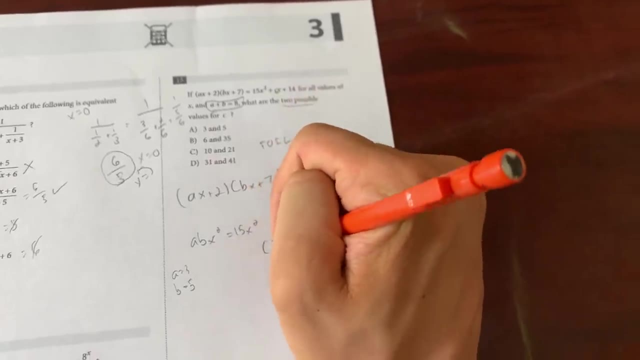 So you have to pick two numbers that, when added together, give you 8 and when multiplied together, give you 15.. So 5 and 3 works fine, Alright. so now we have 3x plus 2 times 5x plus 7. 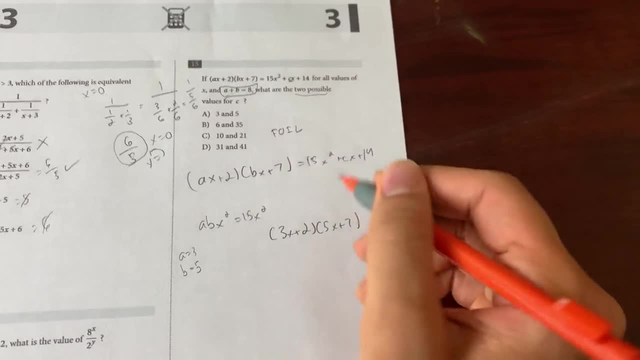 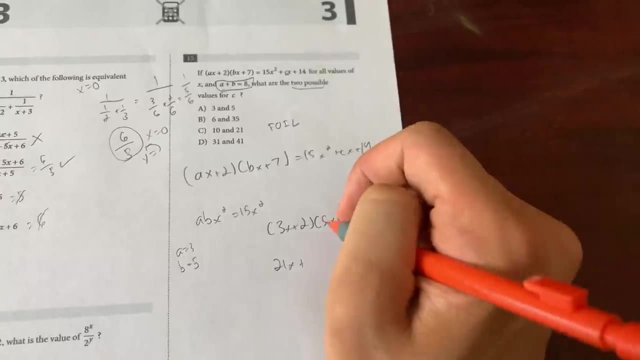 and now we need to find the middle term. In the middle term, all you have to do is multiply the outer and the inner. So let's multiply the outer So you get 21x, plus the inner is 10x, which is 31x. 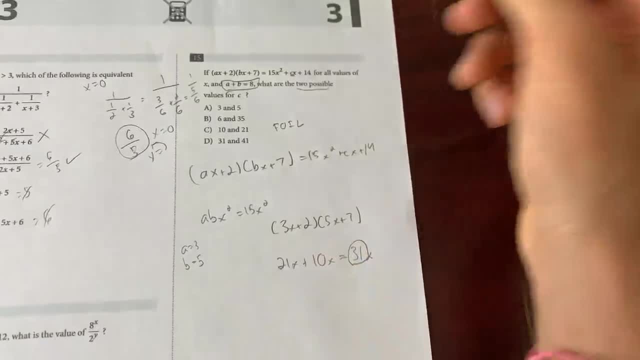 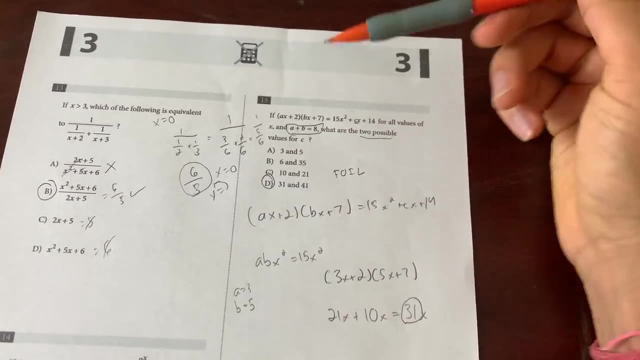 Okay, so one possible value of c is 31.. Bang, Only one of them have 31.. So I'm picking d and moving on. I don't even have to check for the second c value. All you have to do is check for 1. 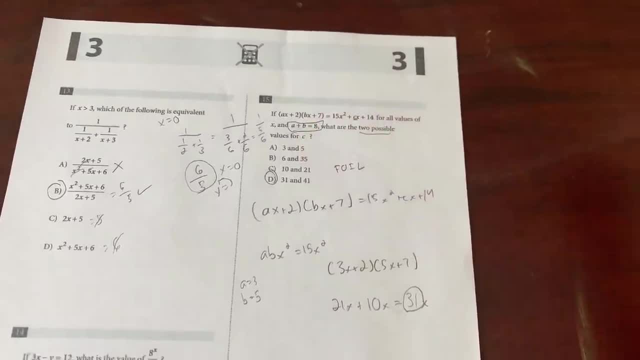 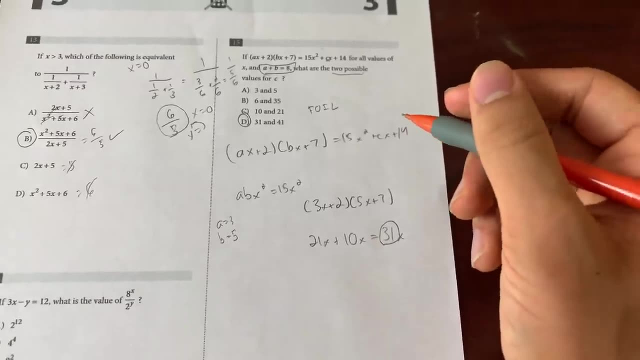 and you can see, none of these have any overlapping values. So once you find one of them, you can move on to the next problem. Of course, if you want to double check it, then you can always just flip it. So now a equals 5. 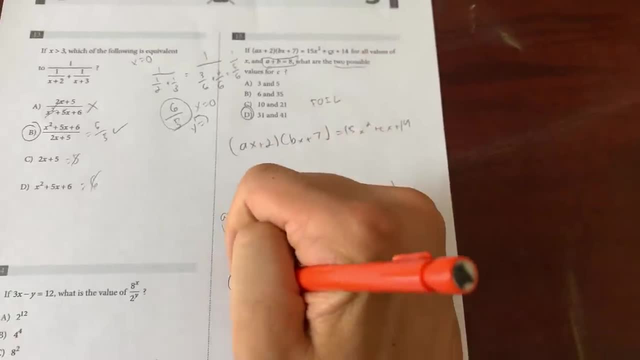 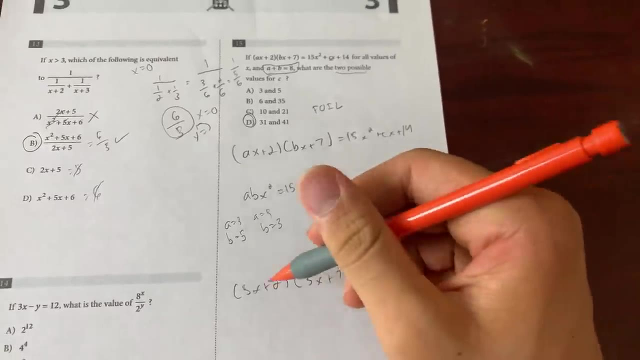 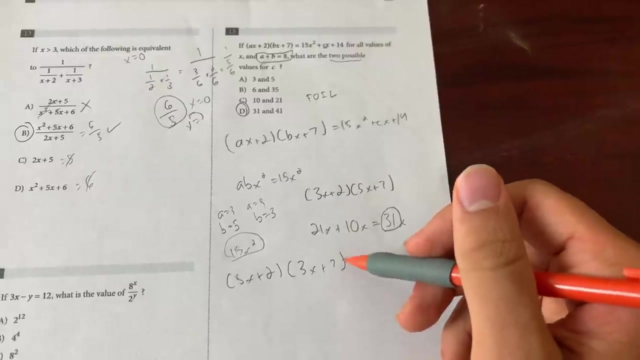 and b equals 3.. In that case you would do 5x plus 2 times 3x plus 7, So in the middle term again 15x squared, because that's the criteria. The middle term was 5 times 7. 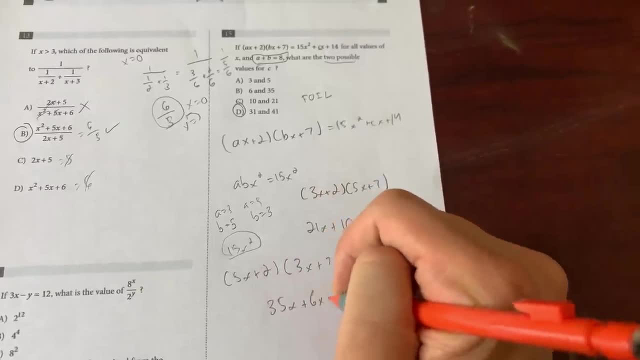 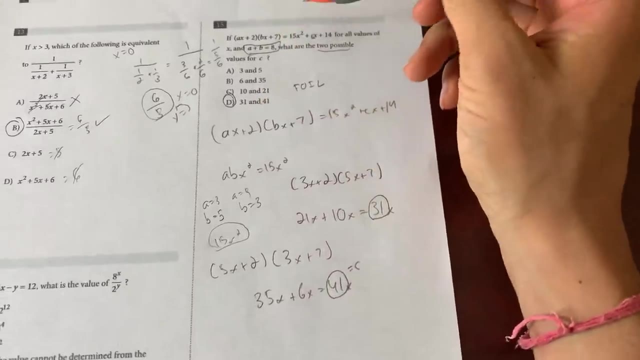 You get 35x plus the inner term, which is 6x, which gives you 41x. So 41 equals c, So 31 and 41 are your two possible values. So see how I deciphered this problem down. 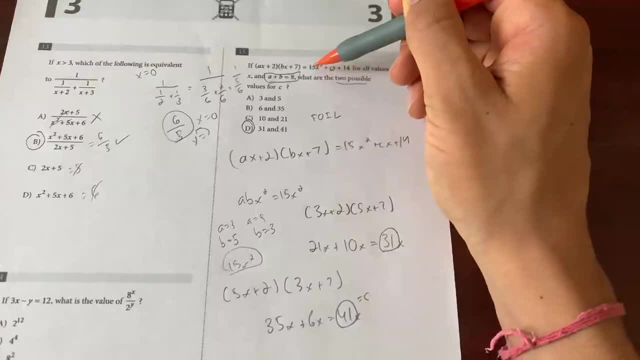 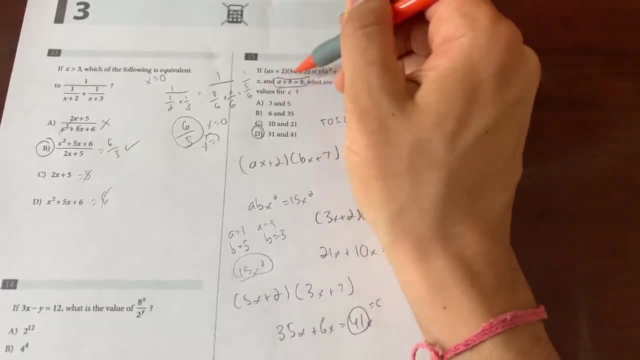 Yeah, it's worded weird. It's kind of confusing the way they word it. If you break it down, you know that it's the same equation. So how can I get this 15x squared? How can I get this 15x squared to appear on the left side? 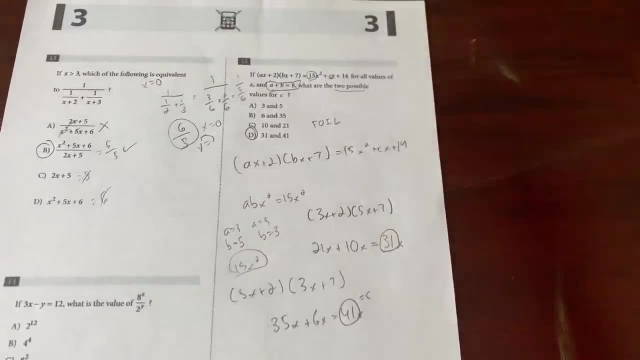 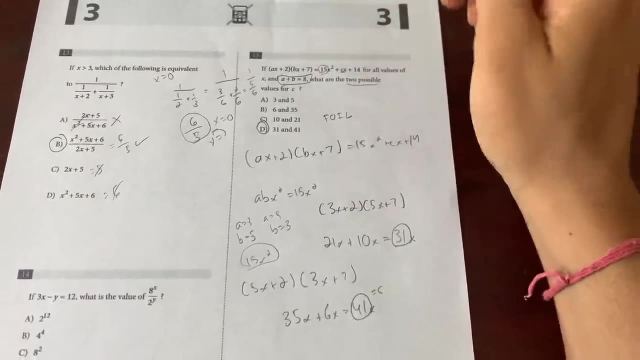 Just make a equals 3 and b equals 5, or make b equals 3 and a equals 5.. And boom, you got it. That's the type of thinking you guys need to have. Work with the problem, Always go to your fundamentals. 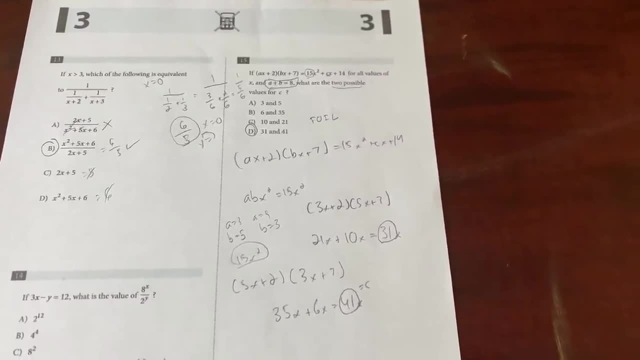 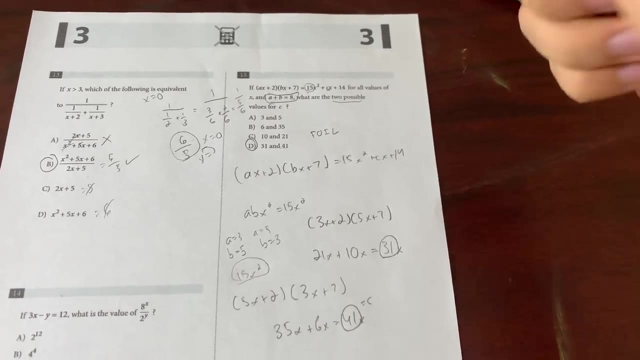 Every SAT math problem. if you've studied and done every topic on Khan Academy can be done pretty easily. I know some sound confusing, but as long as you use your fundamentals you'll be straight. That's all for today, guys. Peace.